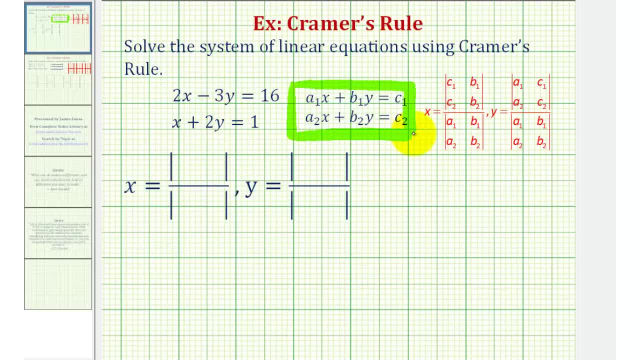 are in standard form or this form here The linear equations are in this form, then the solution or the value of x and y that satisfy both linear equations is given by the quotient of these two, by two determinants. Notice that a sub one and a sub two are the coefficients. 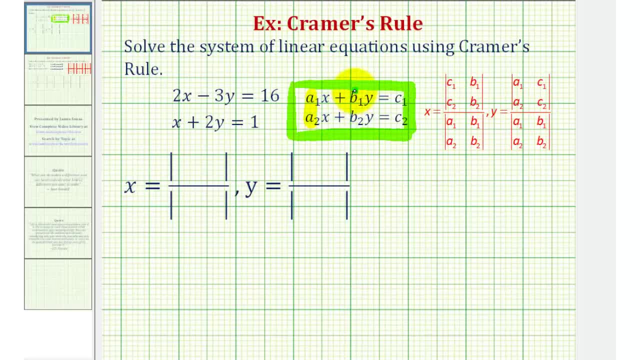 of x, b sub one and b sub two are the coefficients of y and c sub one and c sub two are the constants. So if we take a look at these two by two determinants, let's first focus on the denominator of both x and y. Notice, both two by two determinants contain the same elements. 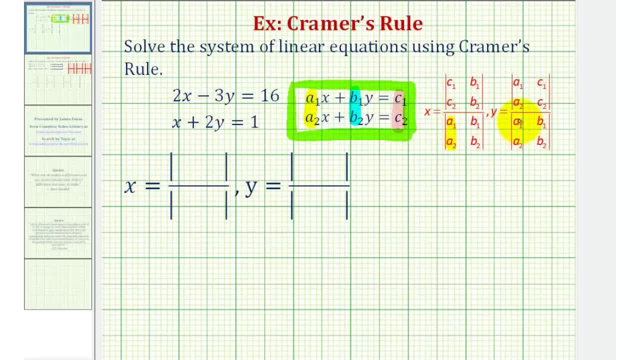 where the first column contains the coefficients of x and the denominator of y. Notice that the second column contains the coefficients of x and then for the numerator of x. if we compare the two by two determinant in the numerator with that of the denominator, notice. 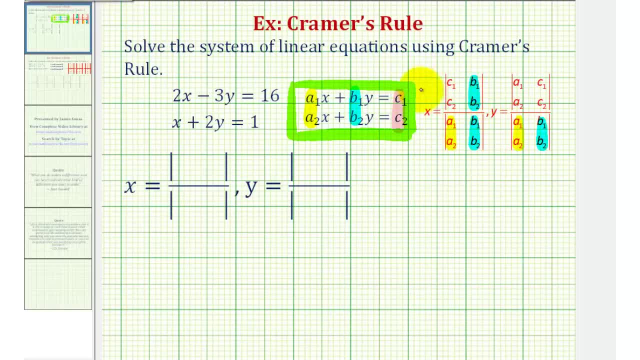 for x. the second column stays the same, but the first column, which in the denominator contains the coefficients of x, is replaced with the constants. So when solving for x in the numerator, we replace the coefficients of x with the constants. Now, looking at the numerator for y and comparing it to the denominator of x, notice that the second column remains an s Record value. 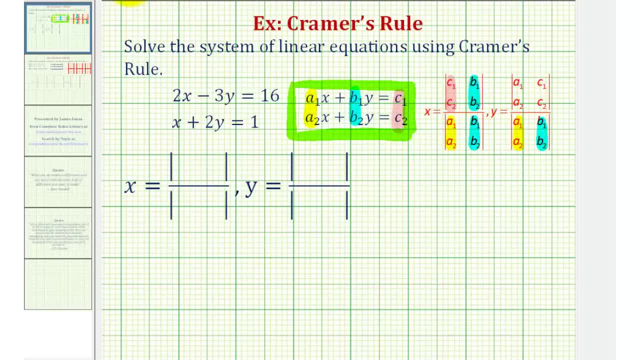 The sum of buying is equal to the sum of their coefficients by the prime of X, x squared times the relevant integral of y denominator. notice how the x coefficients of the first column stays the same, but the second column, which in the denominator contains the coefficients of y, is replaced with the. 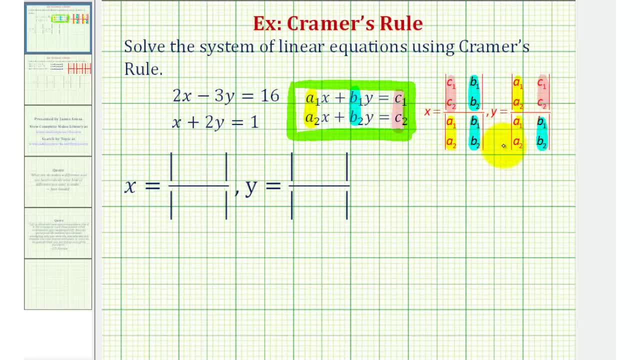 constants. So let's go ahead and apply this to solve the given system, And we'll start by writing in the elements for the denominators for both x and y. So, again using our formula, the first column will contain the coefficients of x, which would be positive, two and positive. 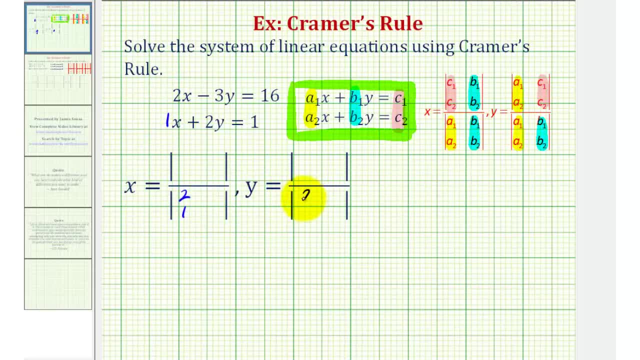 one again for both x and y. And then the second column will contain the coefficients of y, which would be negative three and positive two. And now for the two-by-two determinant for x, if we compare it to the determinant in the denominator. the second column is going to stay the same. And then, because we're solving, 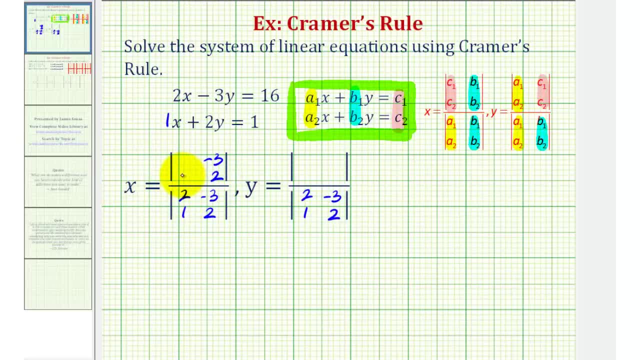 for x, we're going to replace the x coefficients with our constants, which would be sixteen and positive one, And then for the two-by-two determinant in the numerator for y, the first column will stay the same, But the second column, that contains the coefficients of 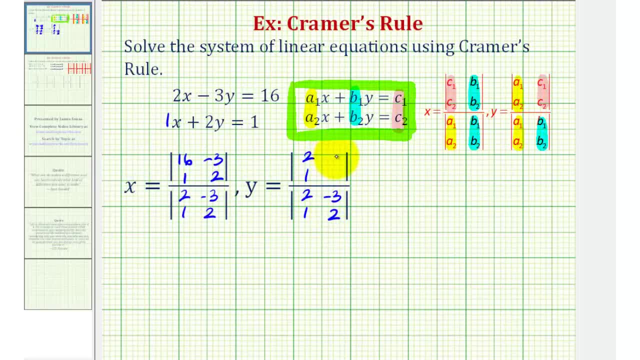 y will be replaced with the constants, so we'll have sixteen and one. Now we'll evaluate these determinants, simplify and we'll have our solution To find the value of our two-by-two determinants. we'll find the difference. 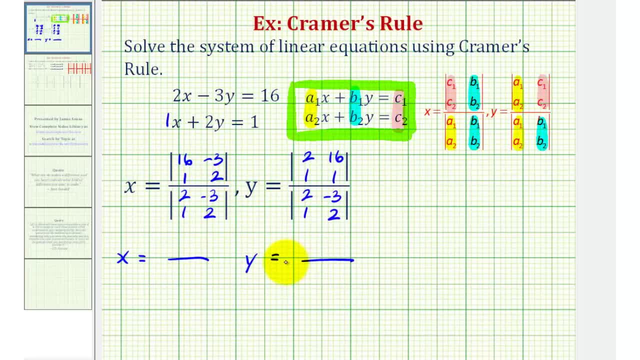 of the product of the diagonals. And let's go ahead and start with our denominators. Here we'll have two times two minus negative, three times one. Well, that would be four minus negative three. Remember this: two by two determinant is the same as. 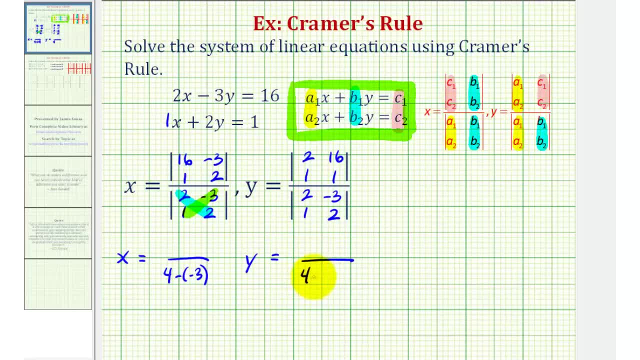 the denominator for y, so we'll also have four minus negative three. The numerator for x, we would have 16 times two minus negative three times one. And then for the numerator for y, we would have two times one minus 16 times one. 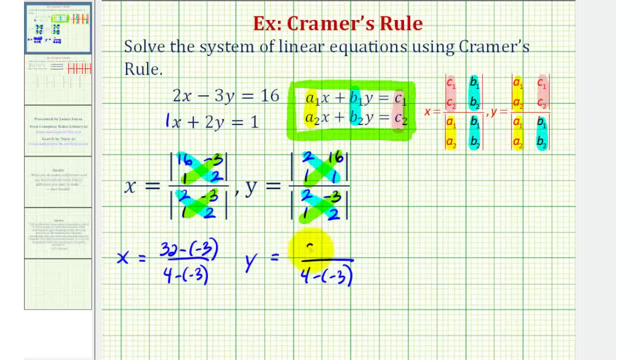 Well, that would be two minus 16.. So we would have: x equals. this would be 35 divided by positive seven, which is equal to five. And for y we would have two minus 16, that's negative 14, divided by positive seven, which is equal to negative two. 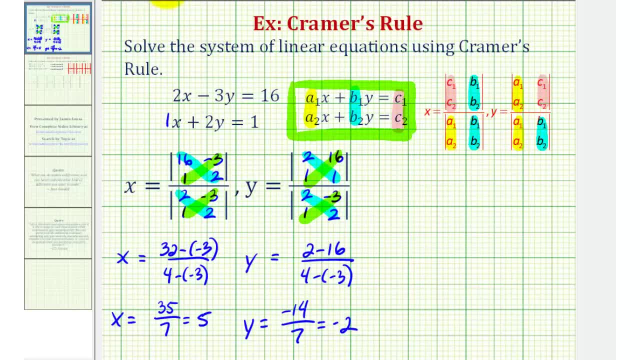 So we can see our system has one solution where the x value is positive five and the y value is negative two. And because our system has one solution, we can say the system of equations is consistent and independent. Let's go ahead and take a moment and check our solution. 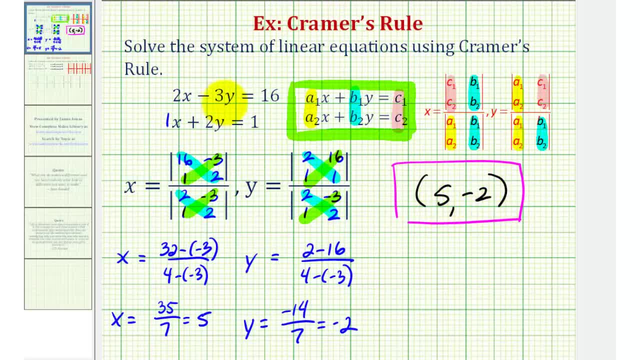 by subbing the value of x and y into both linear equations. So, looking at the first equation, we would have two times x, which is five, minus three times y, which is negative two, equals 16.. We'd have 10 minus three times negative two. 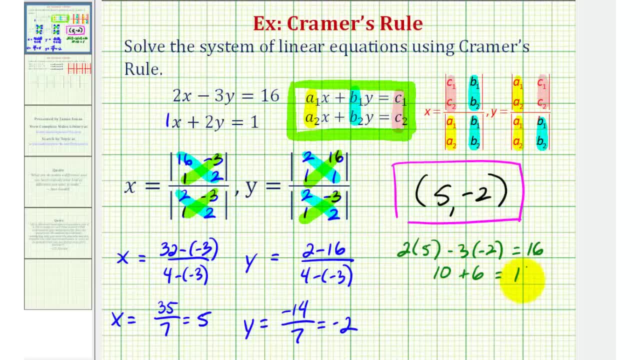 would be plus six, which is equal to 16, so that checks. Let's also check the solution in the second equation: X plus two, y equals one. so we would have five plus two times negative, two equals one equals one. We'd have five plus negative four equals one.